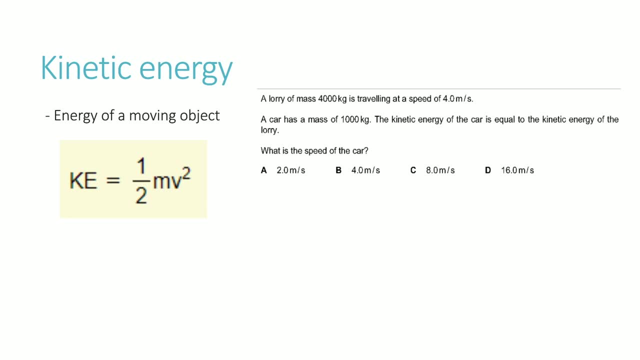 So kinetic energy is simply the energy of a moving object. and how do we calculate kinetic energy? Well, you've got the formula: ke equals half times mass times velocity squared. okay, and so the unit for any form of energy is just joules. okay, so you've got half. you've. 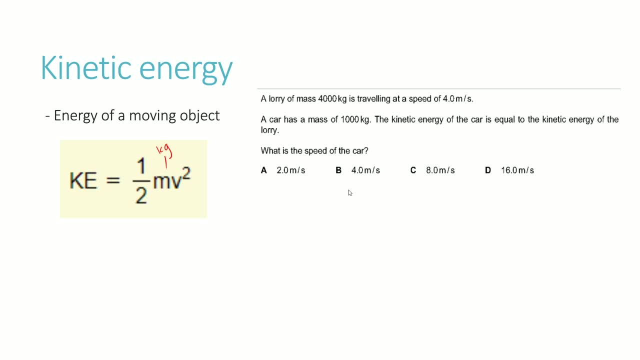 got mass, which is obviously in kgs, and you've got velocity, which is obviously in meters per second. And so when you've got these values that you know, you can calculate kinetic energy. and let's take a look at this example on the right hand side here, which is a very common example. 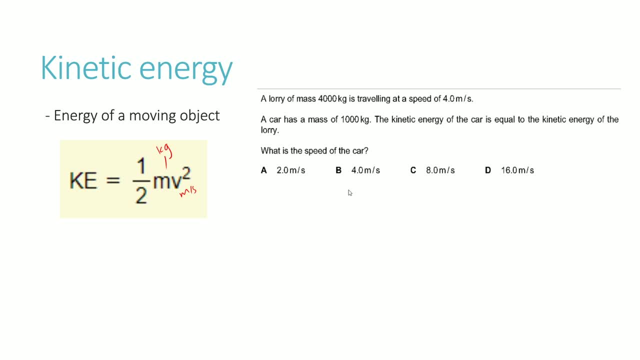 that you'll find in your examination. So a lorry of mass 4000 kgs is traveling at a speed of 4 meters per second. A car has a mass of 1000 kgs. The kinetic energy of the car is equal to the kinetic energy of. 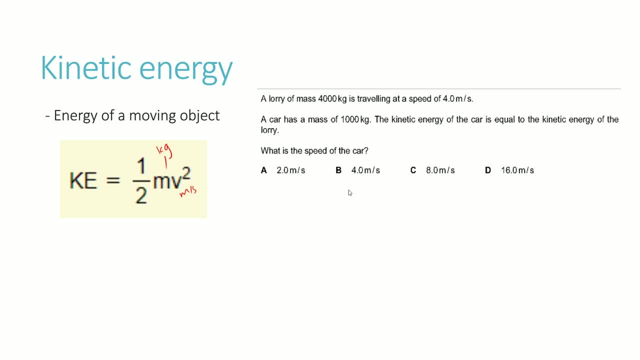 the lorry? What is the speed of the car? Well, we know that the kinetic energy of both cars is at what. We don't know that, actually, but we know that they are the same. So, okay, if kinetic energy of the lorry equals the kinetic energy of the car, what that means is one half times. 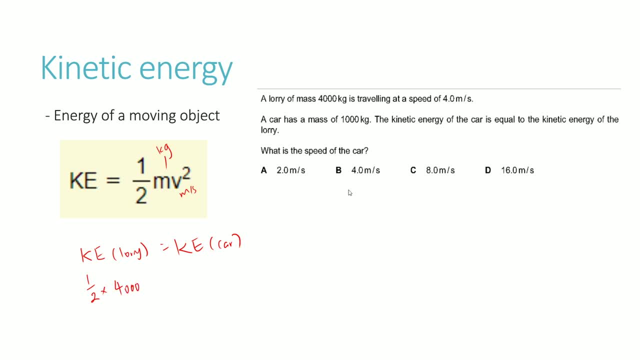 the mass of the lorry times the speed of the lorry squared is equal to half times the mass of the car times the speed of the car. So if you were to simplify that, you've got some 2000 times 16 equals half times 1000,. 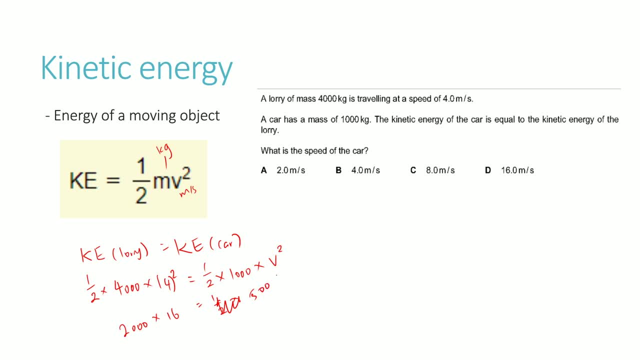 so that's actually 500, times velocity squared. Let me just get the calculator here. So 2000 times 16 is 32,000.. If you want to get rid of the 500 on the right hand side there, well, you've got to do this. 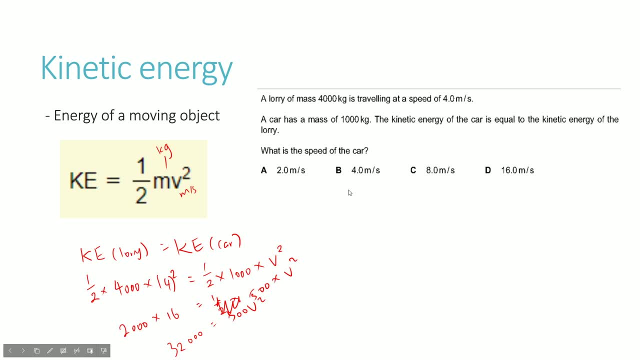 So divide 32,000 by 500, where you get 64.. And finally, if you want to get v on itself, which is the speed of the car, 64 divided by well, 64, square root of that is going to be 8.. 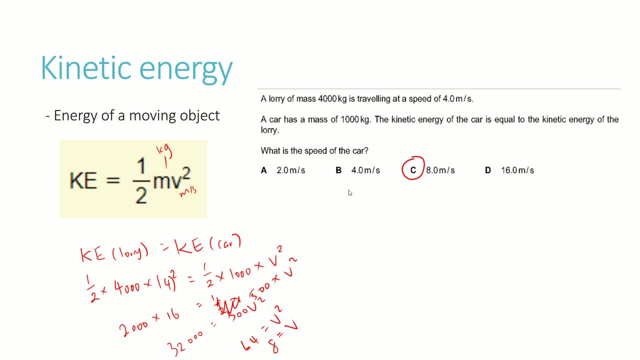 And so therefore, the answer is 8.. So hopefully that makes sense, And so for any object that you have the mass and the velocity, then by using this formula here you can calculate the kinetic energy of any object. So that's a very useful formula that you'll need to know. 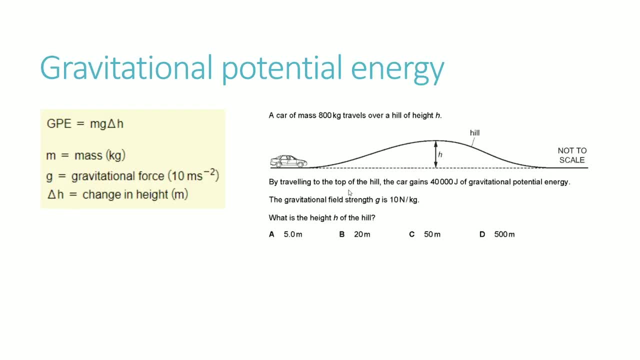 And again, it's always in joules. Gravitational potential energy is also extremely important. And how you calculate that is mass times, gravity times the change in height. OK, So the mass again is in kg. Gravitational force, at least on Earth, is 10 m per second, per second. 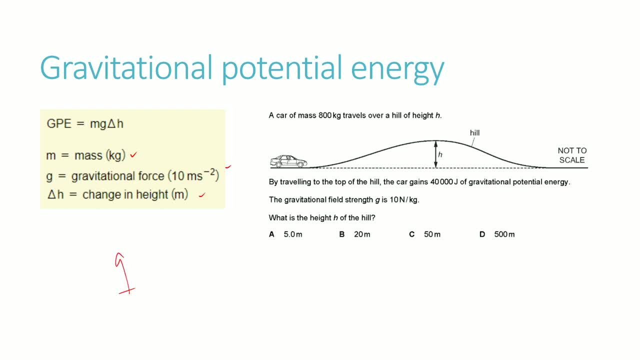 And you've got the change in height, which is how far up are you from ground level? pretty much, So let's take a look at how this might work. A car of mass, 800 kg, travels over a height of h, which is this height here. 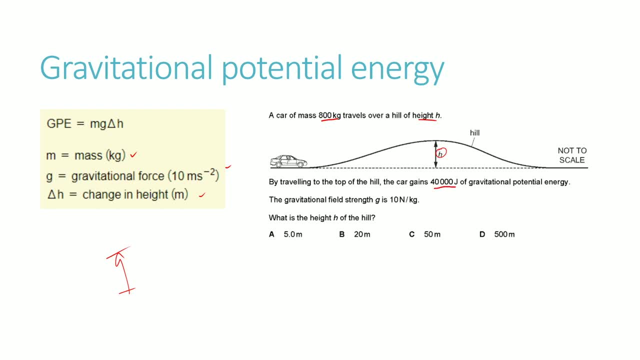 But traveling to the top of the hill, the car gains 45.3 km. 40,000 joules of gravitational potential energy. The gravitational field strength is 10 N per kg. So what is the height of the hill? Let's first of all write down the formula and put: 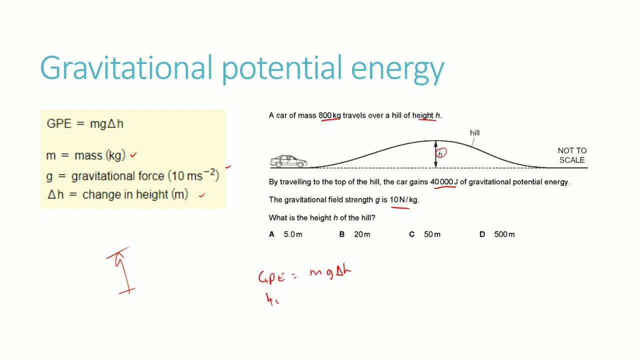 down the things that we do know. Well, we know that it gains 40,000 gravitational potential energy. We know that it's 800 kg, We know that the gravitational strength is 10. But we don't know the height, and that's what we're trying to figure out, Okay, so what you have to do, then, is 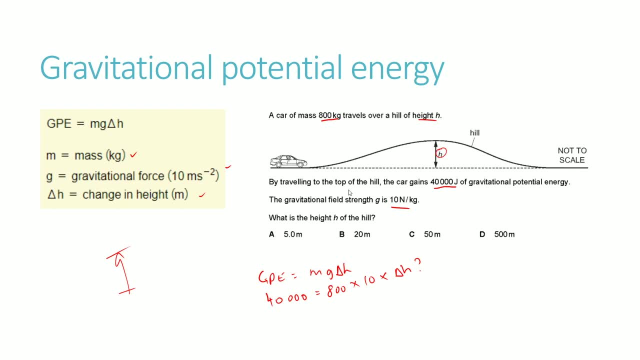 just rearrange the formula. do the calculation. So 40,000 is equal to 8,000 times change in height. So if you were to get rid of the 8,000 on the right hand side, you divide that on the left. 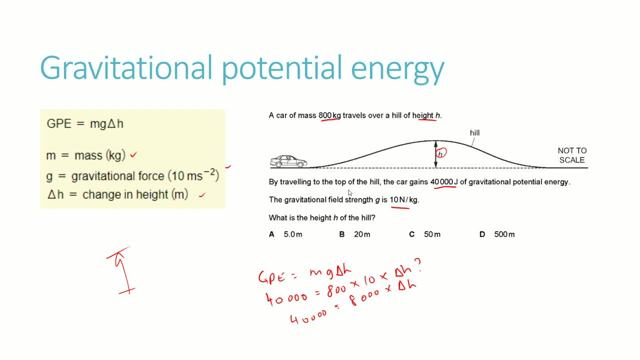 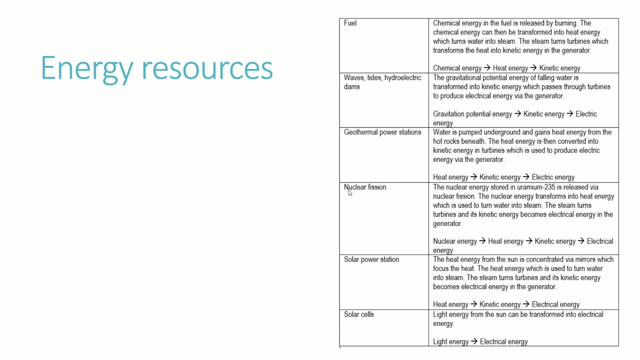 hand side, And what you'll get is 5 meters being the height of the hill. Okay, so that's how you calculate that. So, energy resources: Well, there are many different ways that we can get the energy that we want. A prime example of that would be: how do we get cars to run? Well, we need 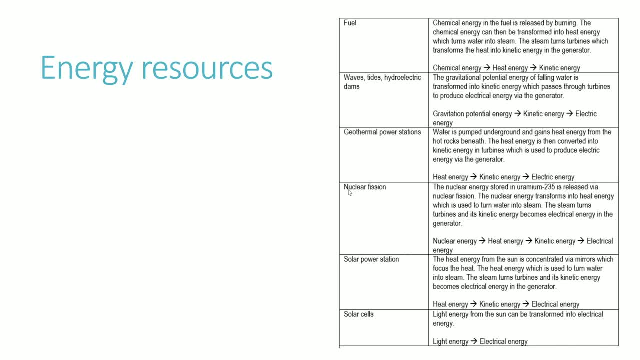 cars. We need cars on the road for transport. How are we going to get that kinetic energy? Well, we use fuel, And fuel is a form of chemical energy that we use When we burn it. what it turns into is heat energy, And so that heat energy then turns into kinetic energy. 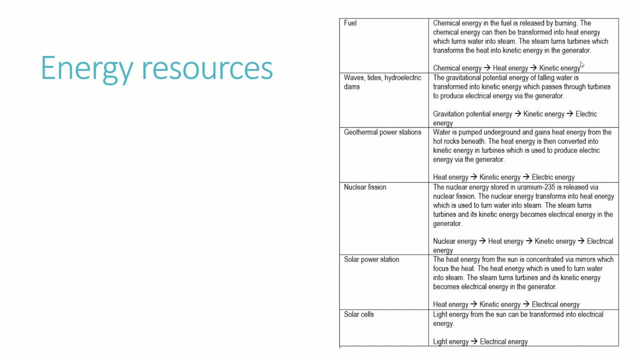 in the form of turbines and things of that nature. So that's one way we can gain kinetic energy, But there's all these other ways. There's all these other things like gaining electric energy with hydroelectric dams and things of that nature. So there's a few things here that we don't really have the time to. 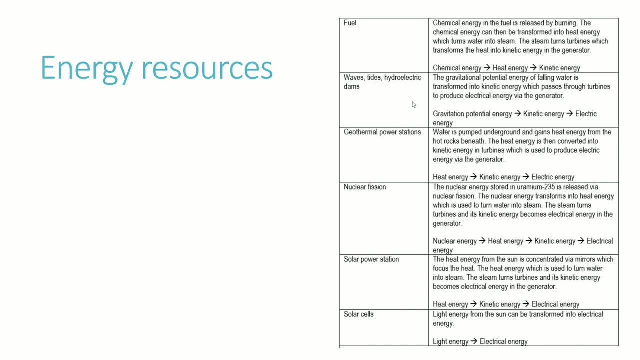 go through, but you can have a read through it. You can also look that up on my website. I've got the same, all the notes- there for you to have a look at, So just have a read through that. So work. Well, what is work? 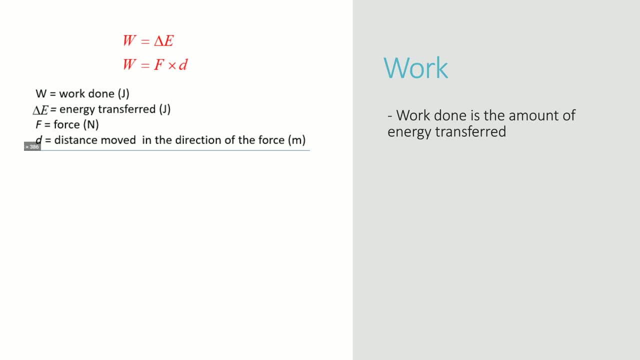 Work done is just Simply put the amount of energy that's transferred in an object, And so how you calculate that is relatively easy. All you have to do is force times the distance that the object is moved in any particular direction. Um, so, if you had like, let's just say a little box here and there's a force of let's. 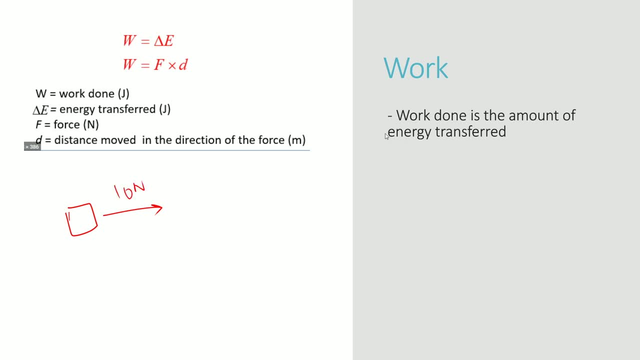 say 10.5.. 10 Newtons going to the right, and let's just say that the distance that the box moved was 0.5 metres, then if you wanted to calculate the work done on this object, it's really just simply 10 times 0.5, which leads you to 5 Joules. 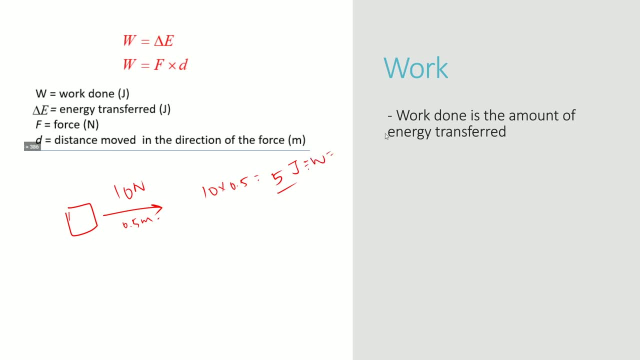 And that's pretty much work, which is also the energy transferred or change in energy. So they're all the same thing. The concept of work is important to consider when we consider what power is, which is basically. the power is the rate of energy transfer, where you know that the energy transfer or the change, 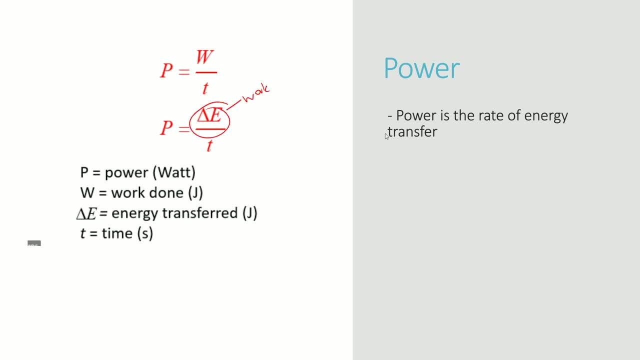 in energy, that's work right. So the rate at which that happens, the rate at which work is done, that is power, and power is calculated in Watts. So, using that same example of that box of- was it 10 Newtons that we had before? 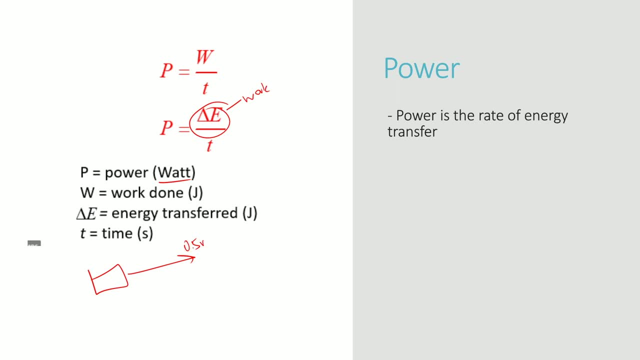 Yeah, okay, it was 10 Newtons, So 0.5 metres have moved and the force was 10 Newtons. Let's just say that this happened over a period of 5 seconds, So what you can do now is calculate the power by going. okay. well, what is the change in? 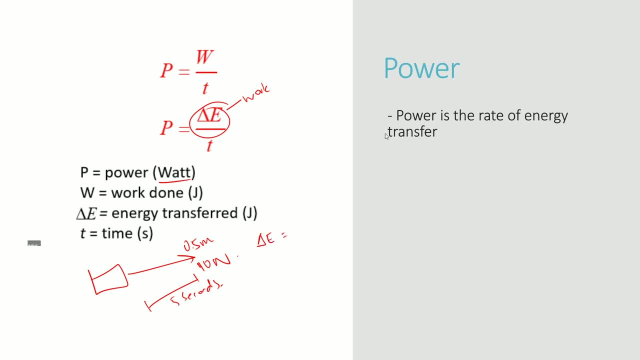 energy. Well, change in energy or work is force times distance, which is 10 times 0.5. so you get 5 Joules. Now what is the power? Well, power is the change in energy over the time period. So you know it's 5 Joules divided by 5 seconds. because you know that's what we're assuming. 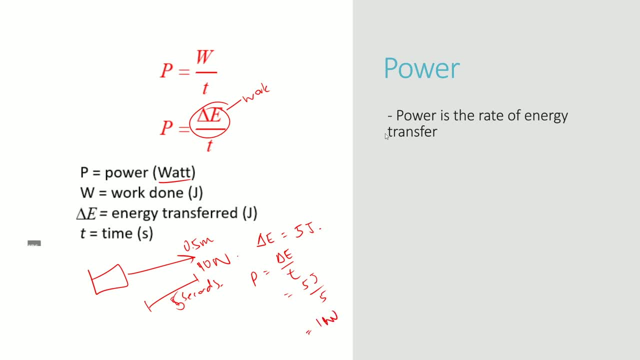 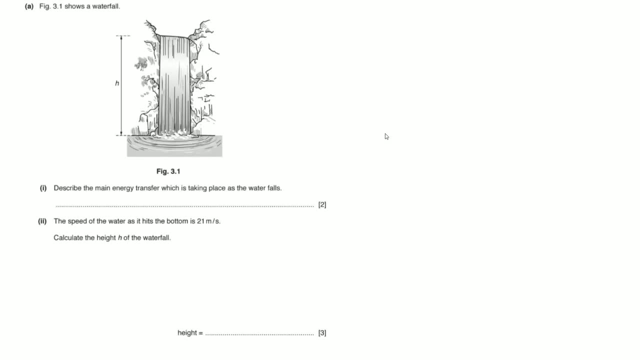 So power is going to be 1 Joules- Okay 1 Watt, Okay 1 Watt. So hopefully that makes sense. So before we finish up, I thought I'd go through this quick example here with you, just to get you familiar with this type of questions they might ask you. 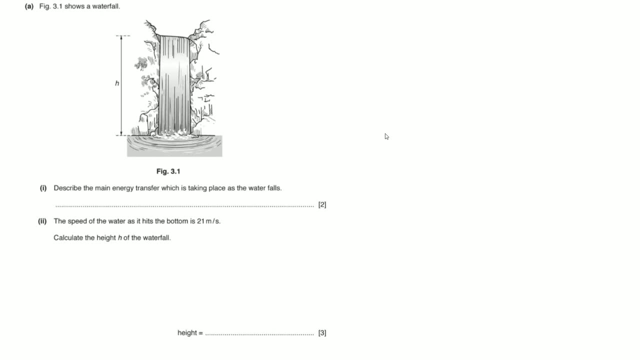 So they give you a waterfall? okay, just remember, the water up here has gravitational potential energy. As it falls down, it gains kinetic energy, and the reason for that is because the gravitational potential energy Is being converted to kinetic energy, And the concept here is that as the object loses gravitational energy, it gains the same. 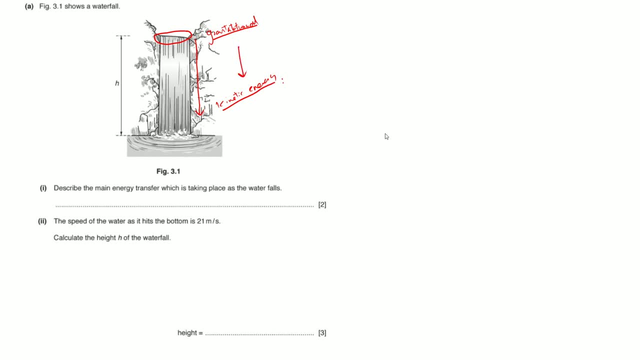 amount of kinetic energy. That's the conservation of energy, where one form simply just you know, gets transformed to another. So the main energy transfer that's taking a waterfall is gravitational potential energy. Okay, So the concept here is going to be: loss of gravitational potential energy is equal to: 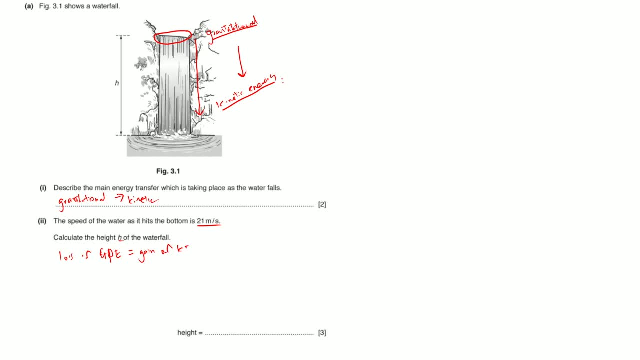 the gain of kinetic energy. Okay, And we know we can calculate kinetic energy because it's half times mass times velocity squared. And we know we can calculate the gravitational potential energy because it's gravity times mass times, change in height, Okay, Now if we were to take a look at this, we know that gravity is 10.. 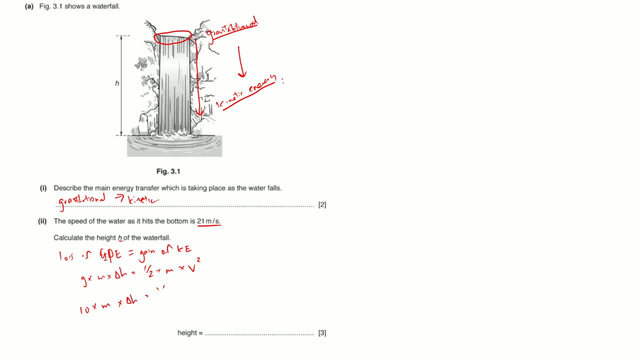 So 10 times mass Times. change in height equals half times mass times. we know what the velocity is, which is 21. And we're going to square that Now. what's interesting here is that you well, we don't know what the mass of the water is. 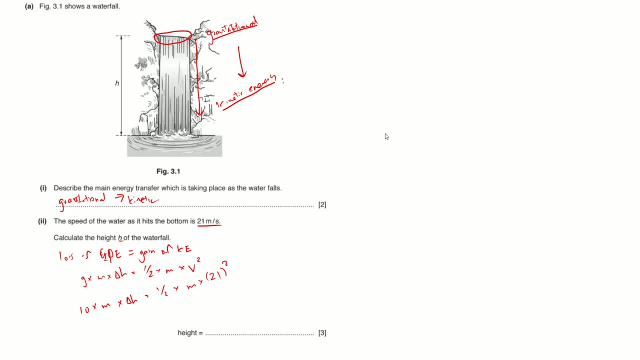 but, quite frankly, we don't need to know, because it cancels each other out. Okay, So we can cancel out the mass. So what you now have is 10 times the change in height is equal to half times 21 squared. Okay. 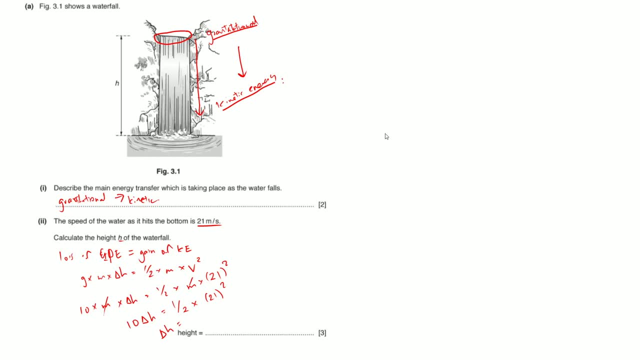 So, finally, change in height is half times 21 squared divided by 10.. And so if you do that- I'm going to grab my calculator- Then what you get is a height of 22.05 meters. Okay So, And so you know, that's one way that they'll ask you questions about this stuff. 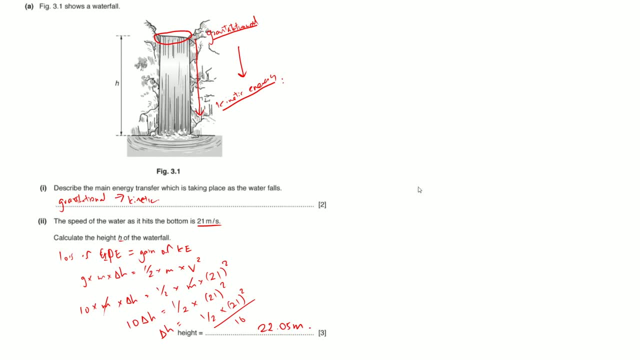 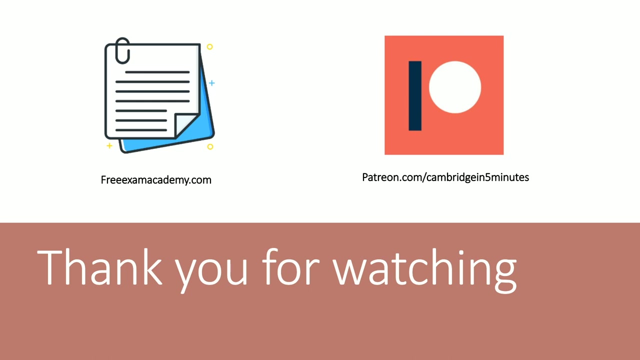 So, you know, just make sure that you're doing a lot of practice on these, because it's quite easy to screw up if you're not thinking right, But it's, you know, relatively straight forward if you practice. So thank you for watching guys. For any extra resources, consider just subscribing to my Patreon channel.